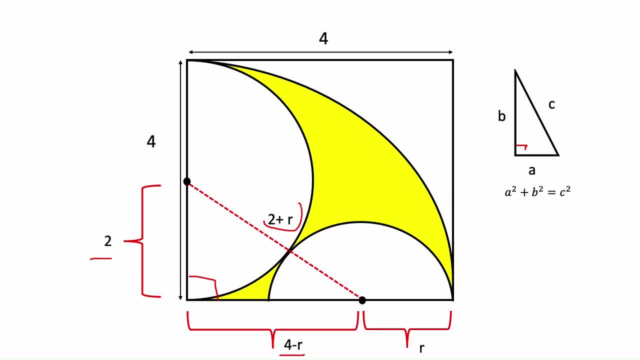 And we know one formula: If we have a triangle with angle with 90 degrees, So it's going to be a square plus b square equals to c square. So we can write this formula for exactly this triangle that we have here And we can find r. 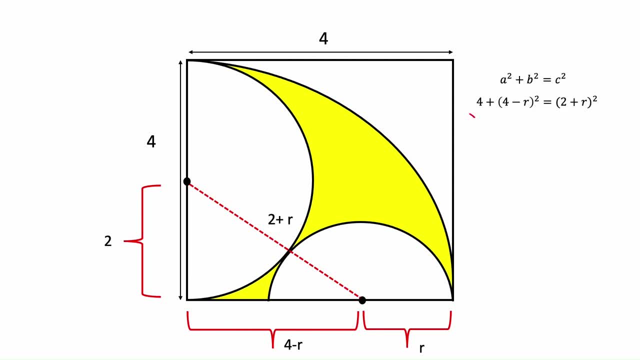 So great. Let's write this formula: It's 2 square which is 4,, 4 minus r square. This is our b And c is 2 plus r square. Let's simplify it: 4 plus 16 plus r square minus, because here we have minus 2 times 4 times r. 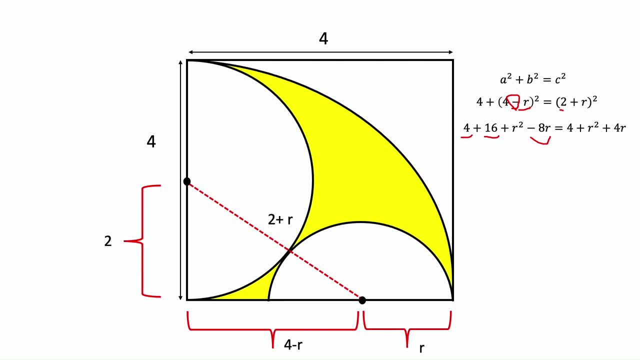 It's going to be minus 8r, And here we are: 2 square, which is 4, r square and plus 2 times 2 times r, which is 4r, And here we want to simplify it. 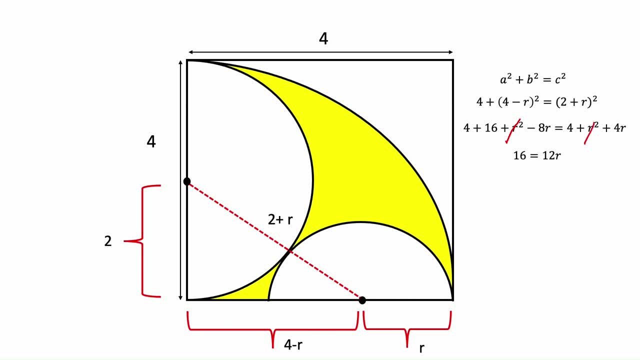 r square will be canceled by r square, And here we have 20.. Here we have 4.. We will have 16 here, And it's going to be 8r plus 4r, It's going to be 12r. 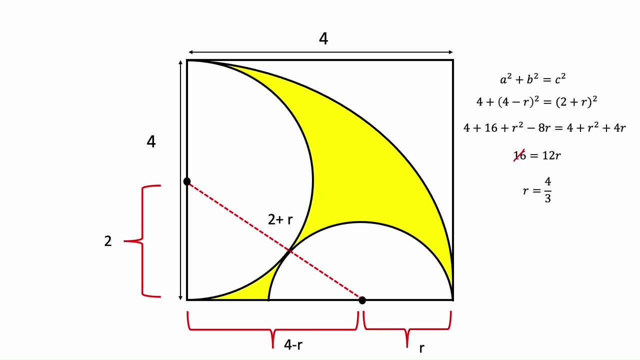 So now we can find r. If we divide both sides by 4, here we will have 4., And here we have 4. And here we have 3.. So r equals 4 over 3.. As I said before, let's assume this is circle 1,, this is circle 2, and this is circle 3.. 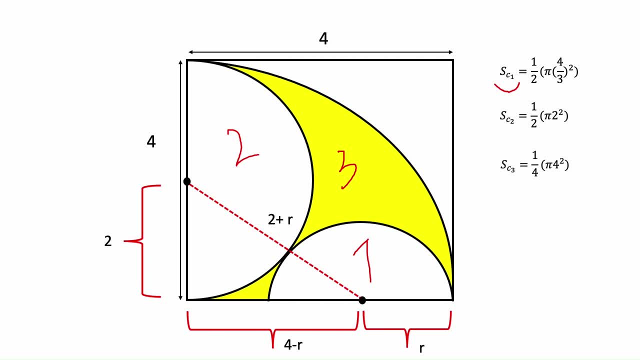 So the area of circle 1 is going to be 1 half, because we have half of the circle, So 1 half times pr square. So our r here is 4 over 3.. So this is our area of circle 1.. 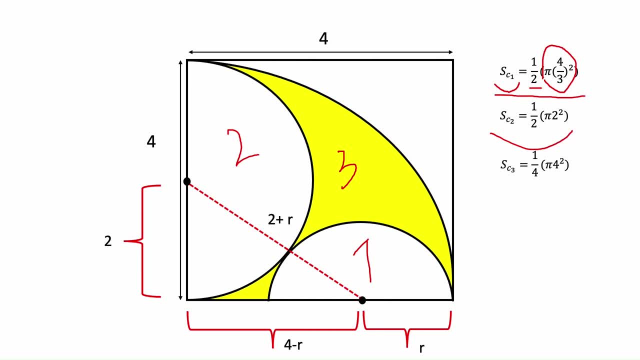 Circle 2 is 4 over 3.. So circle 2 is going to be 1 half again And our r here is 2.. It's going to be p2 square And the area of the last circle is going to be 1 over 4, because it's the quarter of a circle.